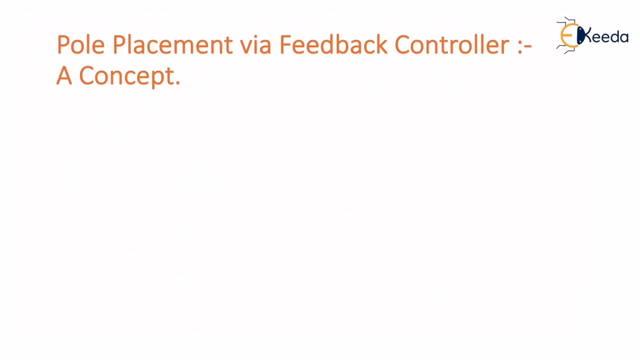 suitable calculations or corrections are been made, and then the transfer function is calculated and, as I said, so it made to obtain a desired specifications. This process of obtaining a desired specifications by manipulating some changes in the gain or pole placement is a concept called as what? pole placement by a feedback controller. Now let us consider a state space model, The. 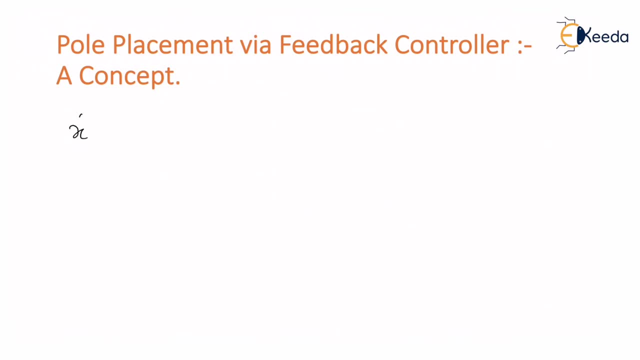 state space model is given, as x dot is equal to a into x plus b into u, and y is equal to c into x plus d into u. This is a generalized state model. This is the generalized state model. Now let us draw a generalized block diagram for the given state model. Now how? 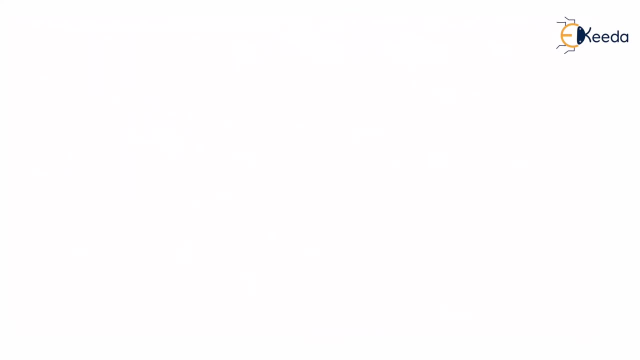 we can draw a block. Let us see So again. for my reference I am taking a model as x dot is equal to a into x plus b into u, and y is equal to c into x plus d into u. So I will first have a summing. 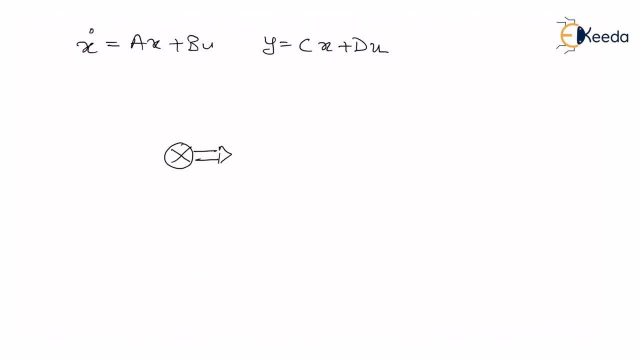 block. Now, this summing block is having a signal called as x dot, which is given as a to a matrix, let us say integrator. Okay, Then the output of this integrator is going to be what: x. Now I will draw a feedback matrix called as a, and this output is given. 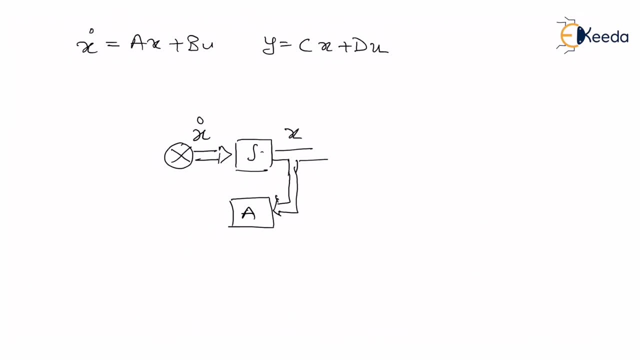 to this matrix a over here, And now it is given to feedback like this: Let us mark it as what Minus over here. So x dot is equal to what Minus a into how much x It is in this fashion: 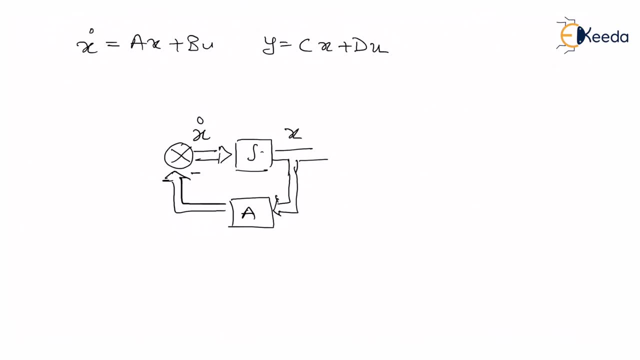 Now, at this moment it is minus a into x. x dot is equal to what Minus of a into x, Like this is the expression. But I actually want x dot is equal to a, x plus b. I need. So what I will do. I will take an input over here. Input is given to a matrix And from this 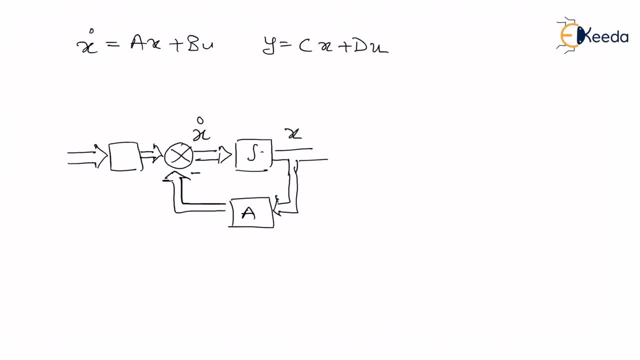 matrix. I am giving to this summing block, So I am making here as plus Again. I am making here as what Plus. Now this sign has been changed, I will make it b over here. Okay, And I am having an input called as what? Let us say u. So what is the expression? now My 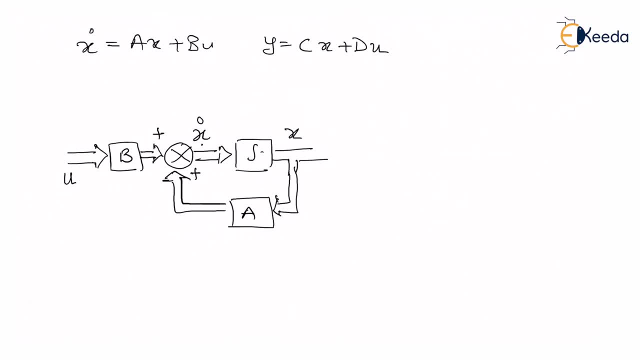 x dot is equal to what. So x dot is equal to a into x plus b into u. Now let us concentrate on the y expression. Y is what c, So I am already having x over here. I will give it to what c. So c into x. Again, I am. 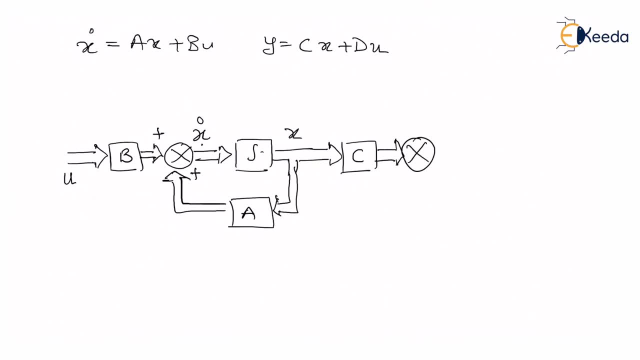 having a summing block over here. Okay, This summing block is having what Plus d into u, So u. I will take a typing from this u matrix or u point. I will get it multiplied with a matrix called as what d And it is given to the 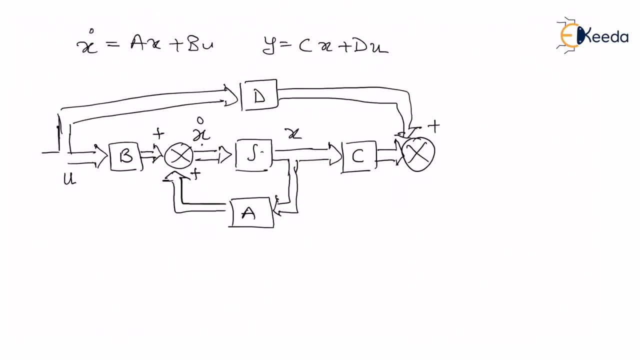 Input part like this. So again I am having plus over here. Again I am having plus over here. So if you look properly, this is given as a output called as what y. So y is equal to what It is, c into x and d into what u Like this. So if you look at the point, my 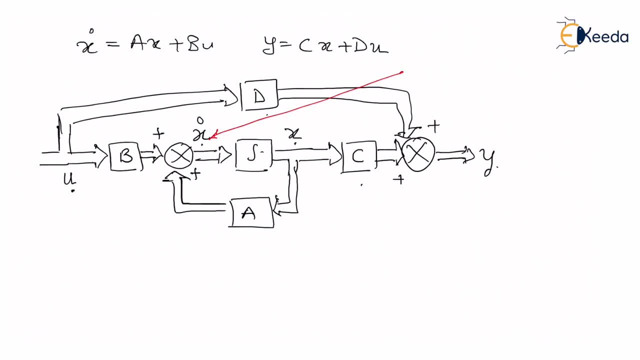 expression for x becomes, or you can say: x dot becomes A into x plus b into u. And for y it becomes: y is equal to c into x plus d into what u. So this is how the state model block diagram is being made. Okay, Done, Now let us proceed. 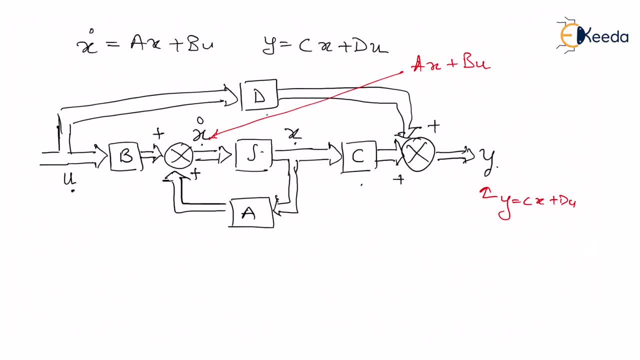 for the next point. What is that next point? Next point is I need to change the pole location. B matrix is what Input matrix, C is output matrix And d is what Direct transmission matrix. I am left out only with one option That is called as what A matrix. Before starting, 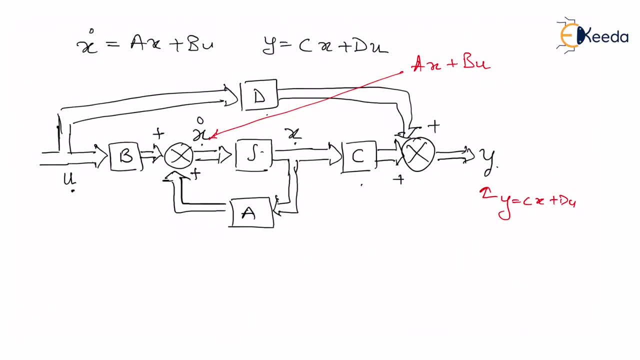 the status of the designing of state space model. I have told you that A matrix is a matrix where we get to know the characteristic equation of a transfer function, where we get to know the pole location of the given transfer function And with the help of pole, 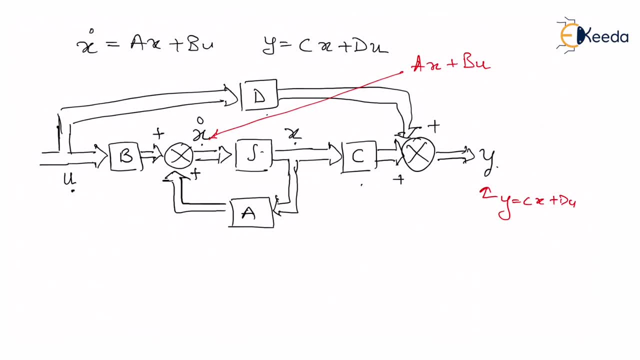 location, I can say whether the system is stable or not. So this is the basic significance of the A matrix, along with B, C and D matrix. B same as it is. So what am I going to do now? Please check carefully what I am going to do now. 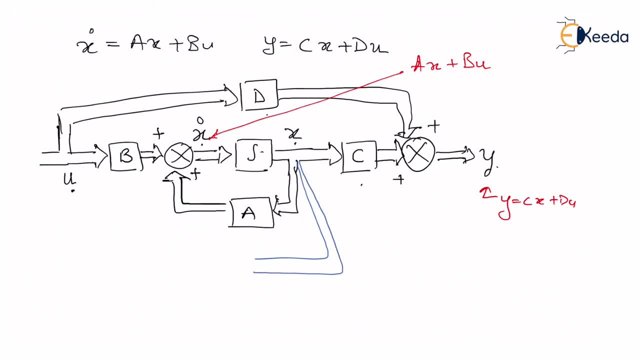 I am going to take a typing from x, I am going to give it to a feedback matrix called as what, Let us say k, Which is given as what Minus, And it is been joined to what U. Okay, So what is the expression? 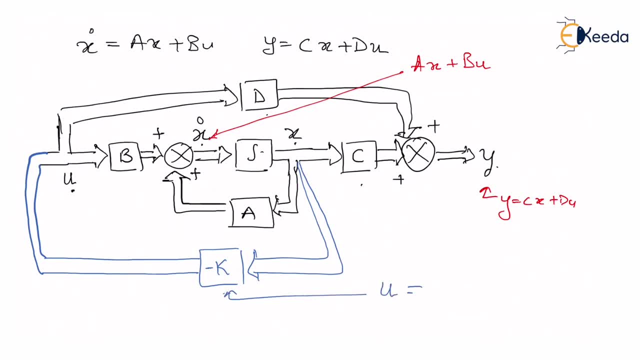 The expression of this k. I can say U is equal to minus k into x. This is called as control law. This expression is called as what? Which law? Control law? Control law expression. Now, what happens because of this expression? A lot thing happens because of this expression. 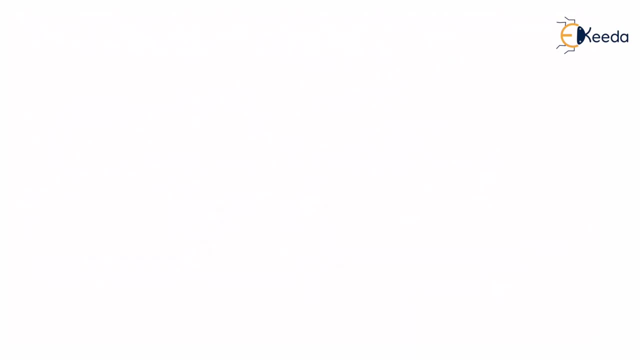 How? Let us see now. Initially, my state model was: x dot is equal to A into x plus what B into U, Yes or no? Now what am I going to do? I am going to substitute: U is equal to what Minus k into x, Yes or no? Okay, So x dot is equal to what A x minus B k into. 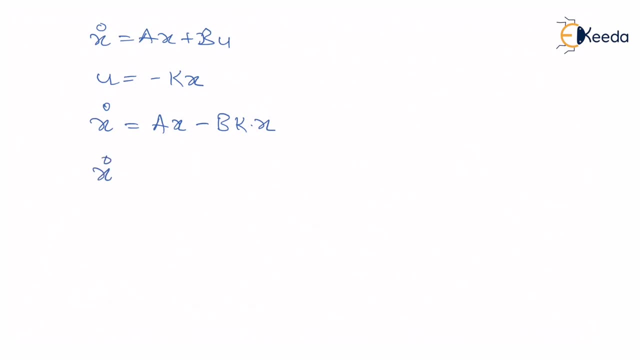 what X? Correct? Okay, So x dot is equal to. Now this becomes A minus B k, The whole common with what X. Now, if you compare expression number one and expression number two, you will get the number two. What change do you obtain? The A matrix is being replaced with. 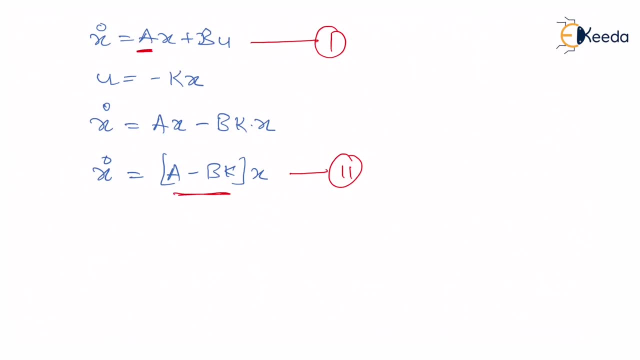 what A minus B k matrix. Okay, This is a very, very important grip of the problem. That is, Jo mera pehle, A matrix, tha The matrix which was A prior has now become as what A minus B k matrix. This is very, very important. So what is the characteristic, equation, Characteristic? 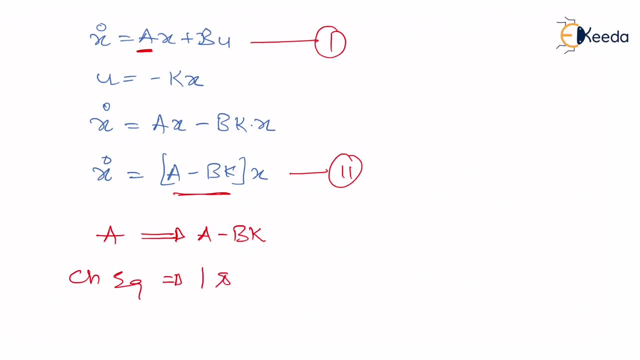 equation was in the form of determinant of S. I minus A is equated to what A minus B k matrix. This is the characteristic equation. Characteristic equation was in the form of it toward 0. this is called as what characteristic equation. now, because of this, a becoming a minus b. 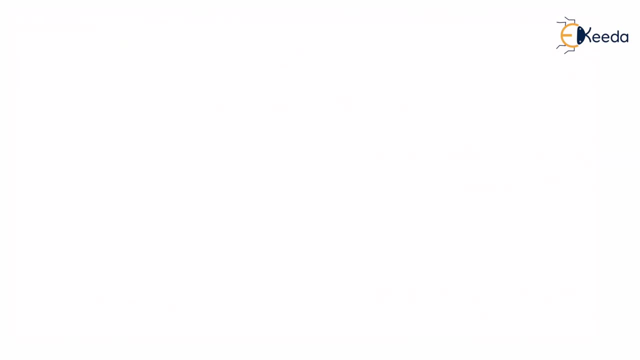 k. the characteristic equation is replaced as follows: it becomes determinant of s i minus a. it was prior like this. now this a is substituted as what a minus b k in the above expression. so what do i get? so i get determinant of s i minus common with what a minus b k, the whole common. 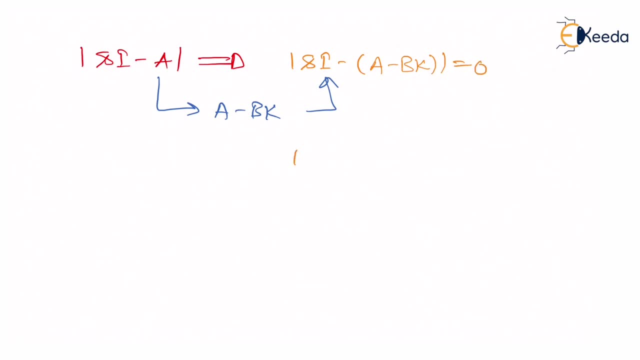 is equal to what 0. if i expand what i'll get determinant of s i minus a, plus b k is equal to what 0. so the new characteristic equation is what it is nothing but determinant of s i minus a. so plus b k is equal to what 0. this is the most grip of the concept that is, a control law or 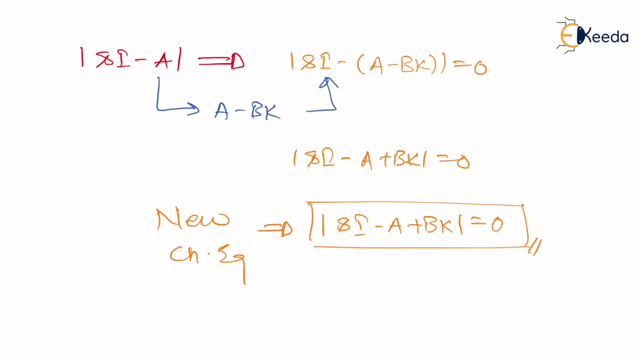 pole placement via feedback controller, that the characteristic equation is being changed with the help of what determinant of s i minus a plus b k. now, in the next session, i am going to discuss the different ways in which we can design or we can solve the problem of control law. just. 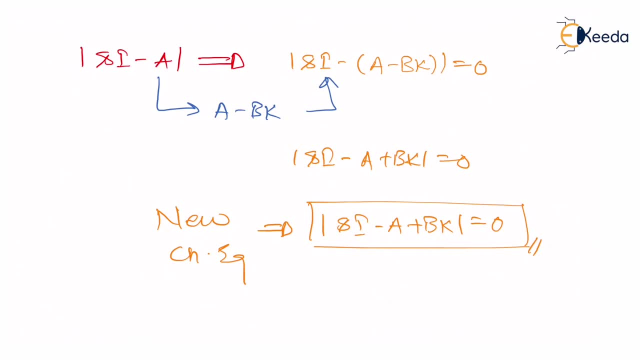 for introduction point of view, i am going to discuss the three methods. the three methods in which the control law can be solved are as follows. methods method number one is called as matching coefficient. matching coefficient method and this is very easy to understand understand. second, Ackermann's method. 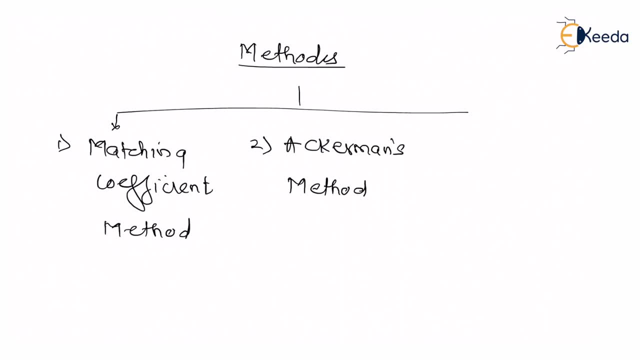 Ackermann's method- again very easy method to understand. and the third is transformation method. transformation method, again very easy to understand. so I have got three methods matching coefficient, Ackermann's method and transformation method. now what am I going to do in my subsequent three different different slides? I am going to